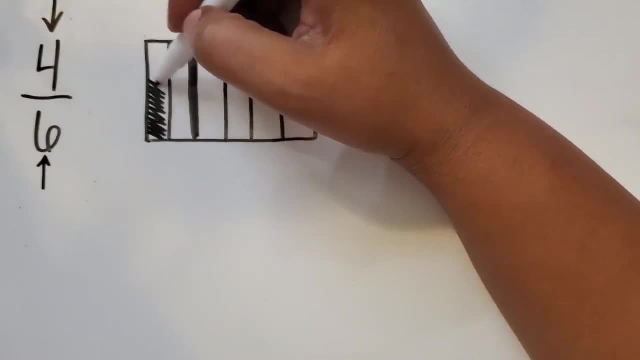 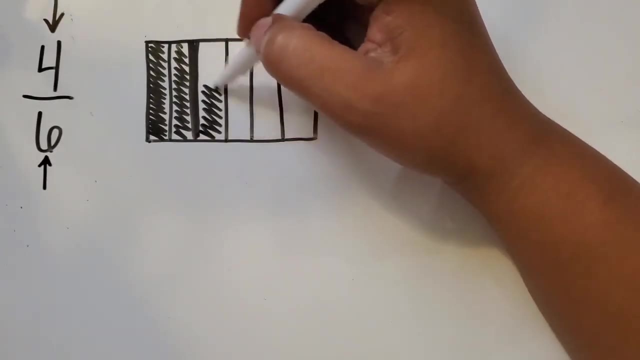 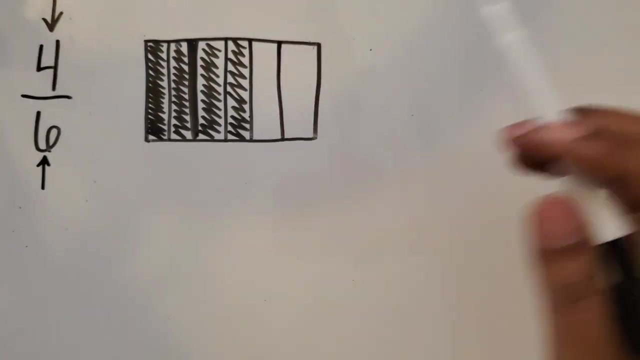 a model Are we going to shade in? So I'm going to draw in 4 of those 6 equal parts. So out of 6 equal parts, we have 4 that are shaded in, and that is representing 4-6.. Let's look at. 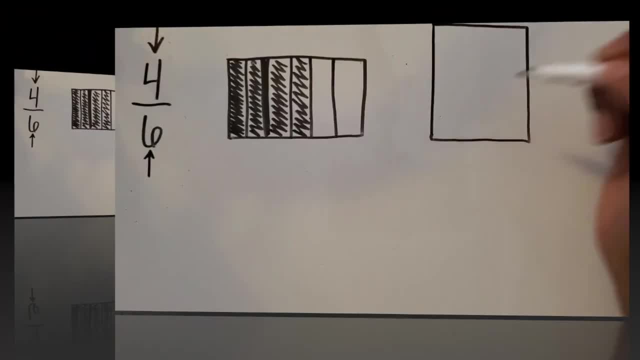 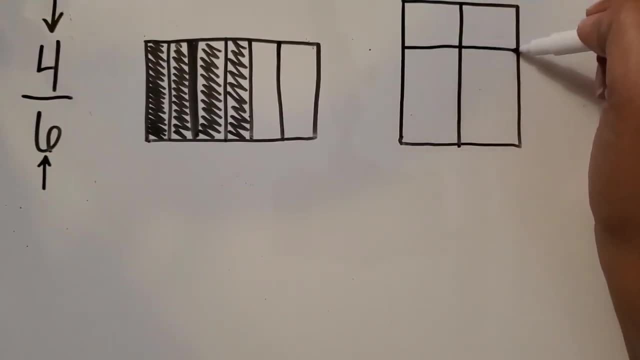 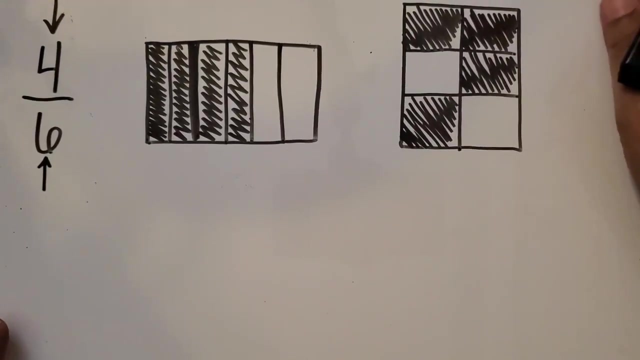 another model we can use to represent 4-6.. Using a different size whole, I can partition my whole in half and then into thirds. So from these 6 equal parts again I need to shade in 4 to represent the fraction 4-6.. So the question here is: does this model still represent 4-6?? Yes, because, as we're, 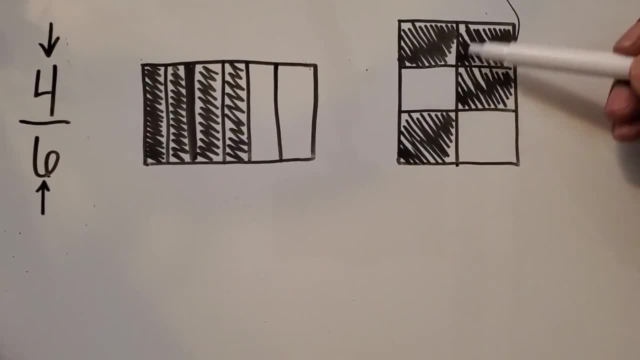 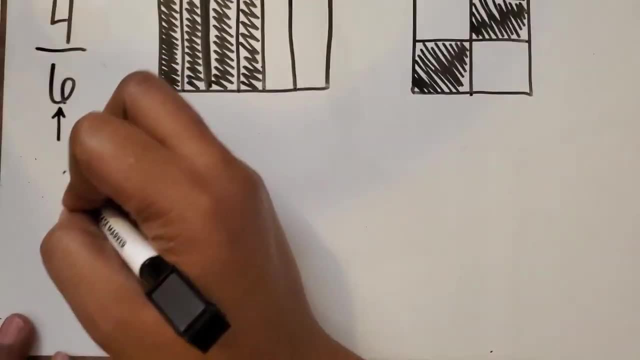 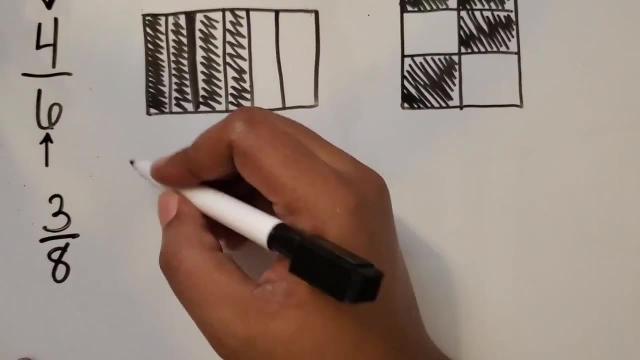 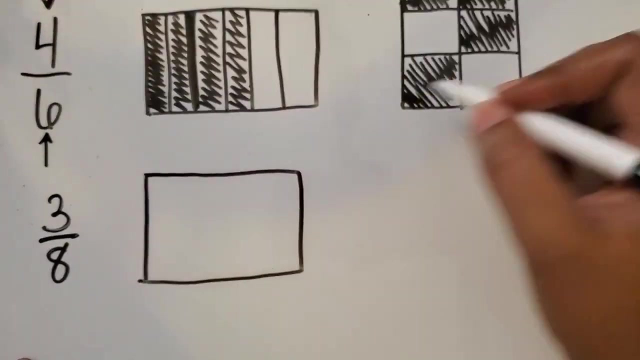 going to draw the whole out of 6 equal parts. 4 are shaded in, even if all 4 are not right next to each other. Let's look at another example. We have 3 eighths. How can we represent that in a rectangular area model? So I'm going to draw another whole and my holes are different. 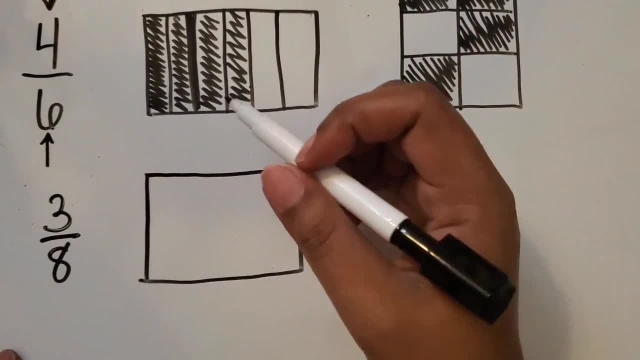 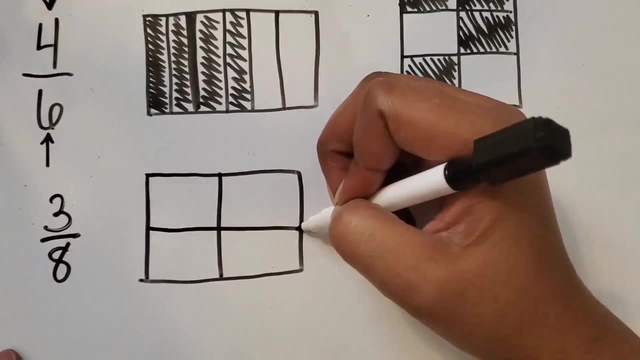 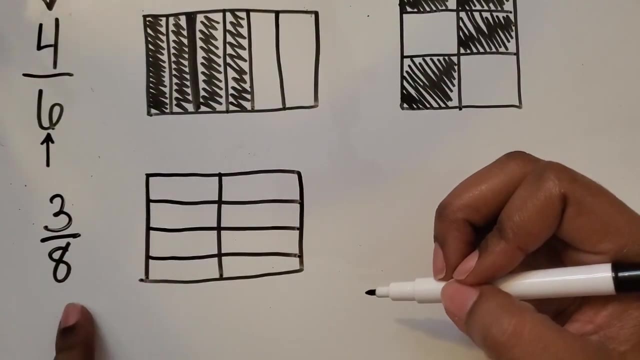 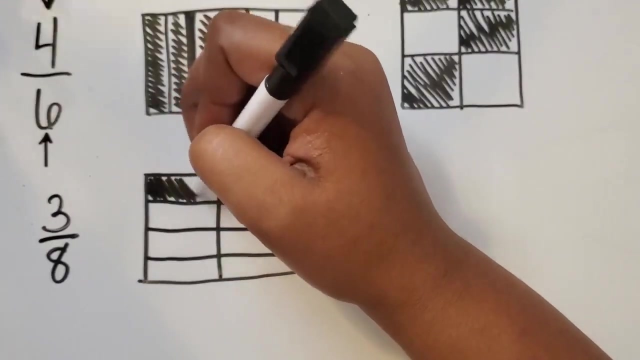 sizes in each example. So for this whole we have 8 total parts, 8 equal total parts, and we need to shade in 3 to represent 3 eighths. So we're going to shade in 8 equal parts. Let's see: 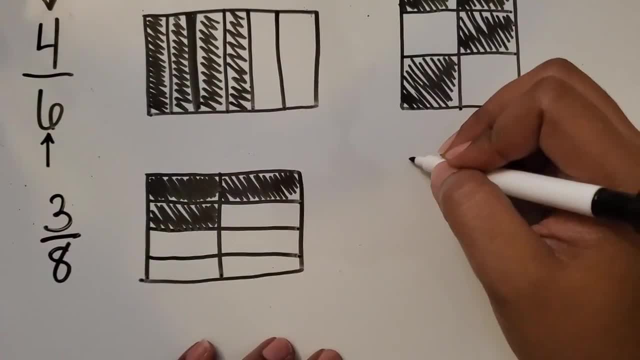 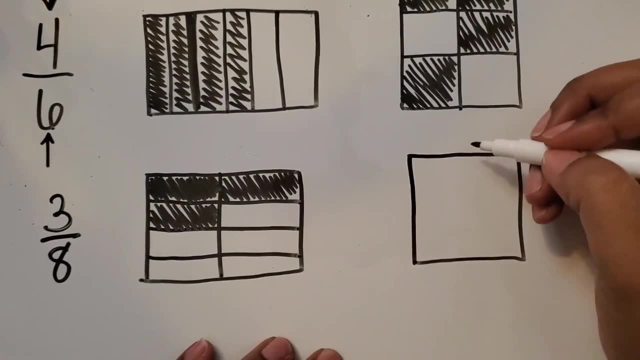 Let's see, Let's see. So for this whole, we have 8 equal parts, 8 equal parts And we need to shade in 3 to represent 3 eighths. Now let's look at one more. So I'm taking that whole. I partitioned it in half. 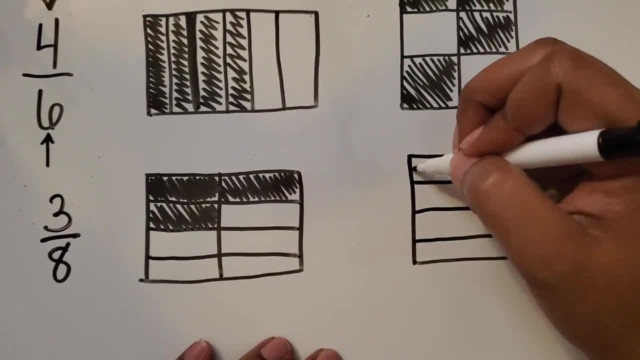 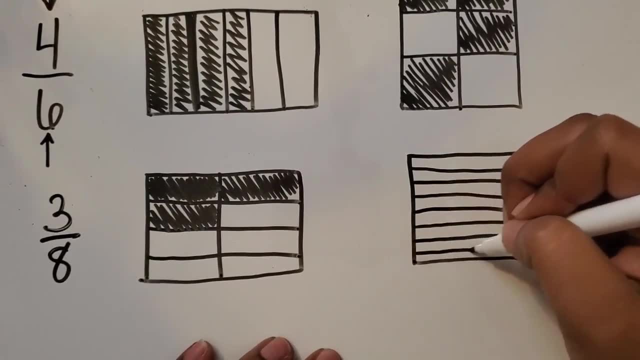 then I partitioned both halves in half to create fourths, and now I'm going to partition each fourth in half to create eighths, because it's eight, eight, there are eight equal parts. Okay, one, two, three, four, five, six, seven, eight. 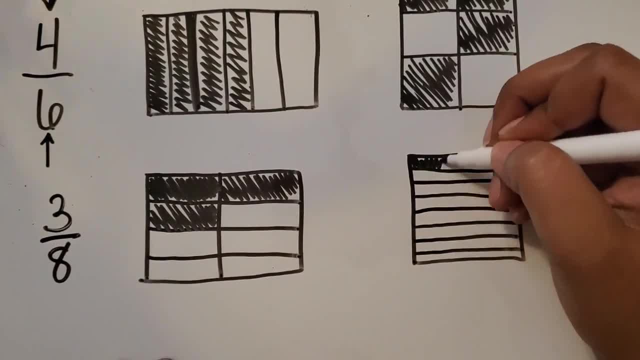 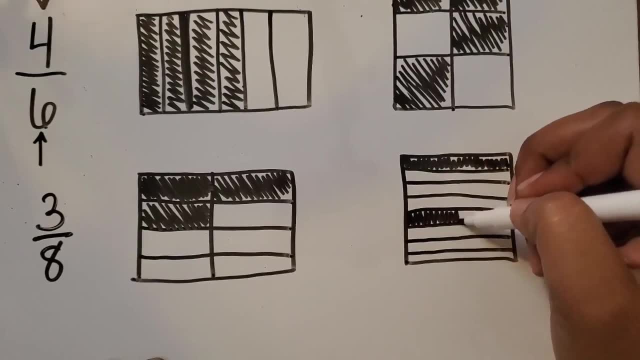 We're going to shade in three of them Again. they can be next to each other or they don't have to be. We just know that out of the eight equal parts, three are shaded in. Now what if we wanted to represent a fraction? 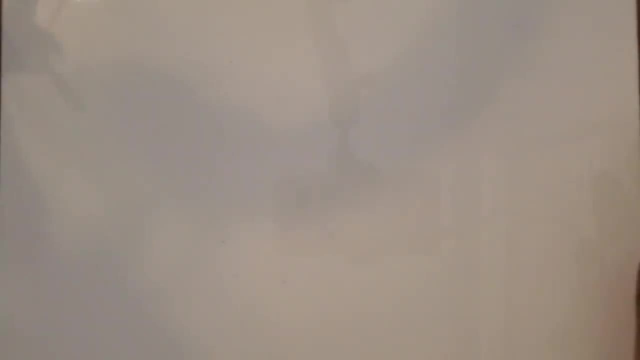 greater than one or an improper fraction. some people know it as using a rectangular area model. So what if we had the fraction greater than one? nine, six And again, it's a fraction greater than one because the numerator is larger than the denominator. 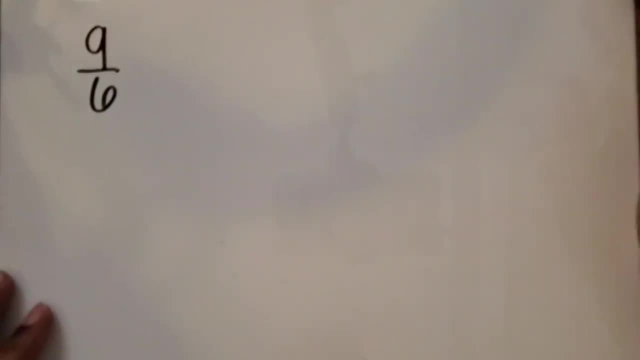 so it has a value that is greater than one whole. So let's think about representing nine, six and a whole. In the last example we saw how we can, how we could, partition a whole into six equal parts, So we're going to do that again. 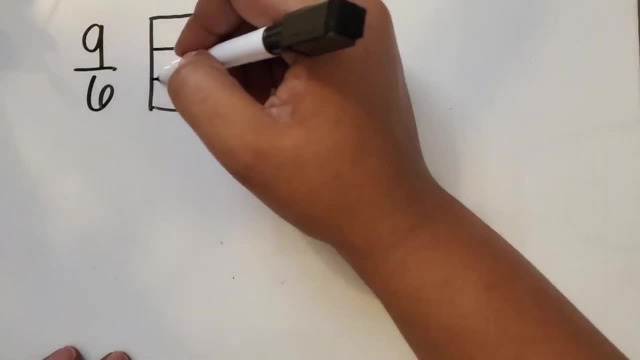 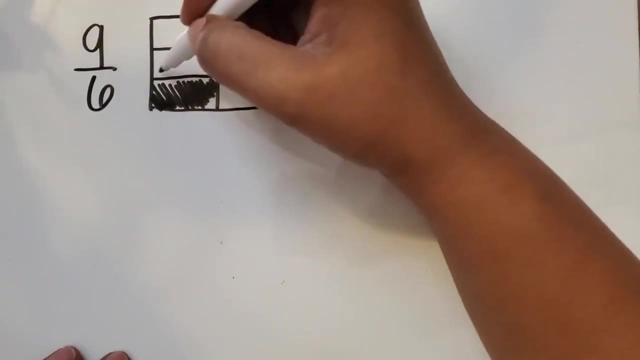 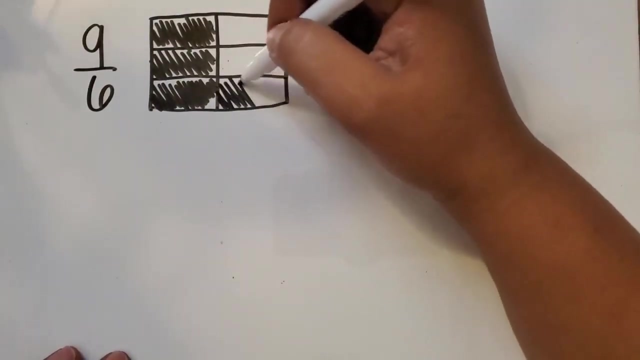 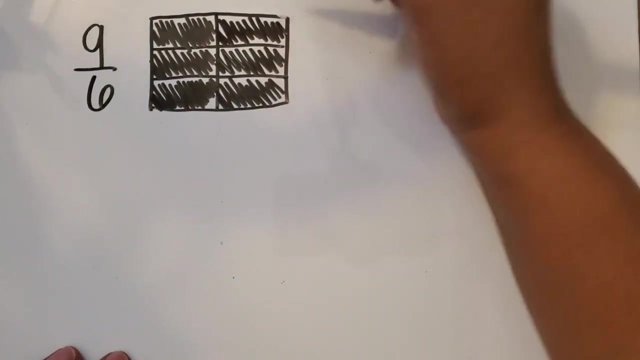 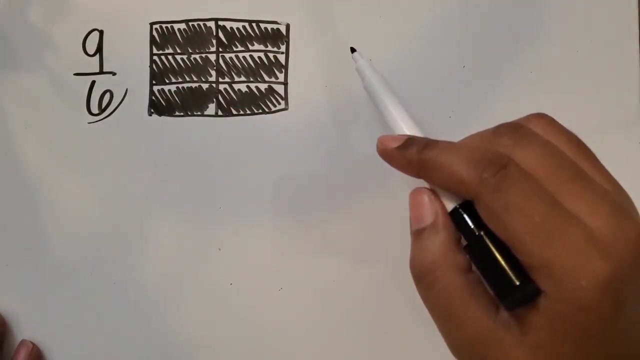 And I'm going to shade in six of those parts. We need six, six to fill that whole. But wait, our fraction, our fraction greater than one, shows nine six. I need to create another whole so that I have enough to show nine six. 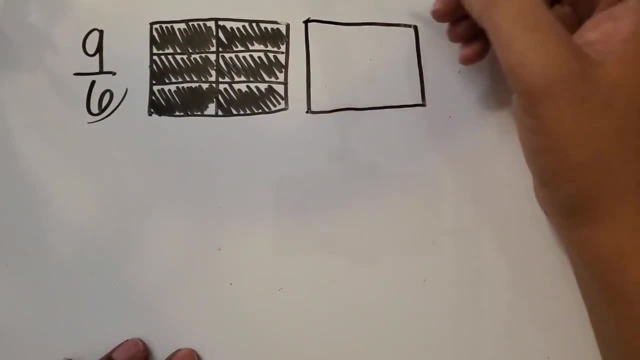 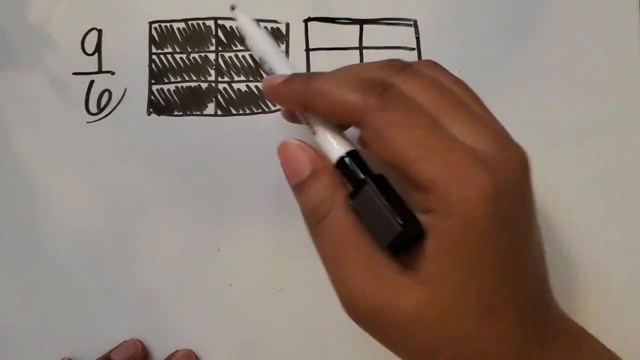 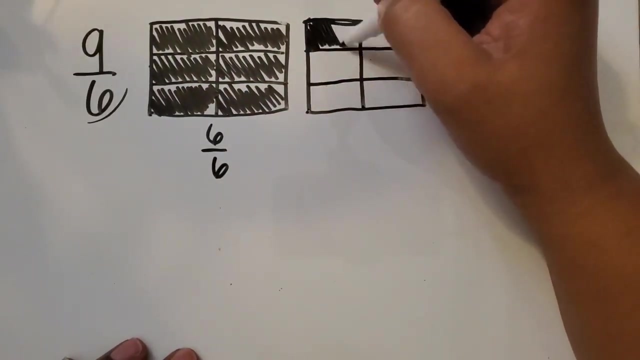 And I want my wholes to be the same size, about the same size. So I already have six, six, we can write that down. I need to get to nine, six. So let's see One more is seven, six. 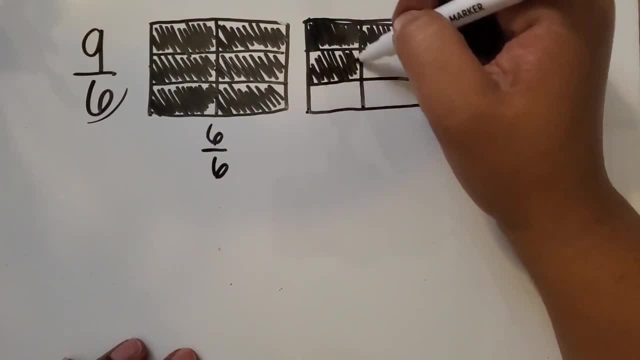 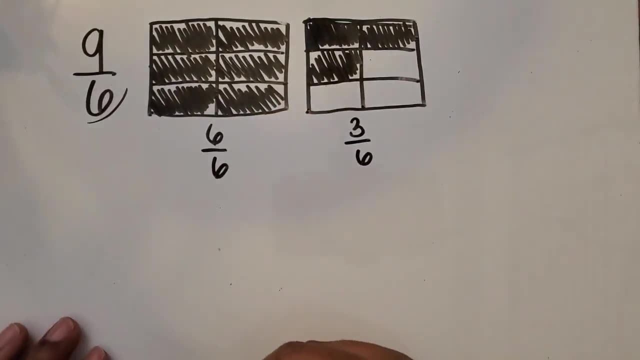 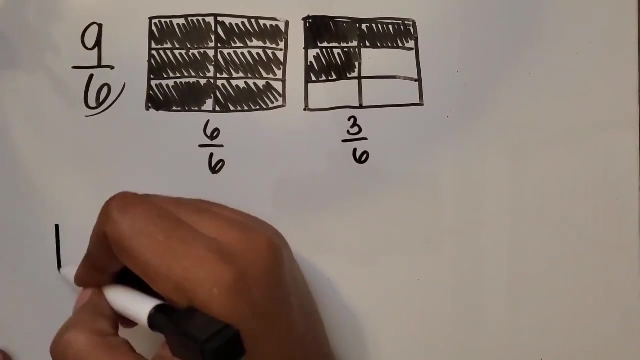 eight, six and nine, six. So we have three, six here and six, six here. together That equals nine, six. Let's do one more example: 10, four. So again our denominator tells us how many.